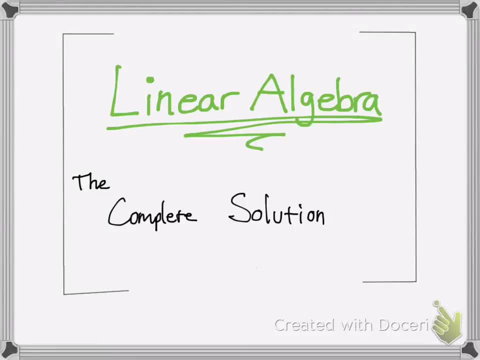 Hello, YouTube. Alright, this is it the complete solution. If you've seen my other two videos on the particular solution and the special solution, well, this is like the culminating thing right now. This is the complete solution, which makes up the particular and the special solutions. 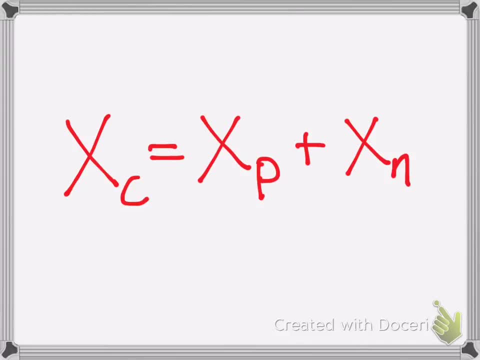 So, again, you've seen this formula in the previous two videos as well. We looked at XP, the particular, and XN, the special solutions, and now we're going to look at XC, the complete solution, how it makes up those two parts, the particular and the special. 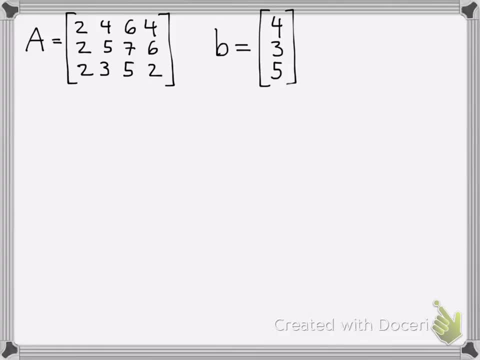 So how do we approach this? Well, we have our matrix and we have our B right, So the first thing we want to do, we'll just start with the row reduction. it's pretty easy. I encourage you all to pause the video and practice your row reduction. 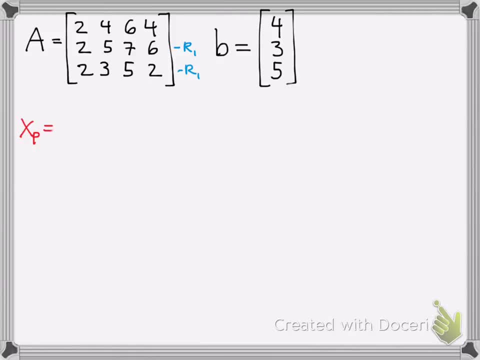 But first we're going to start with the particular solution, Since we have our B already. So what you do to find a particular solution, all you do is augment A with B and continue on with your row reduction. So after you row reduce, we're going to have to do another step here. So we're going to add row 2 to row 3, and you should get this right here. 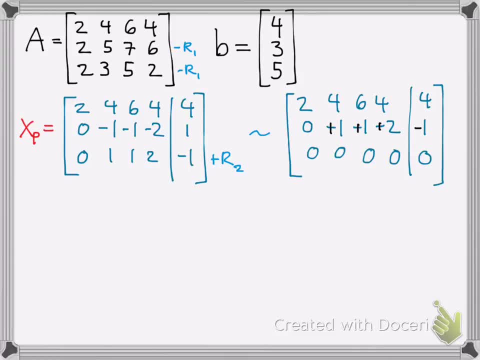 Now, if you notice in the black there I divided by negative 1 to make all the numbers positive and easier in the matrix itself. So I'm going to do that. So I did that extra step just for simplicity for later on. 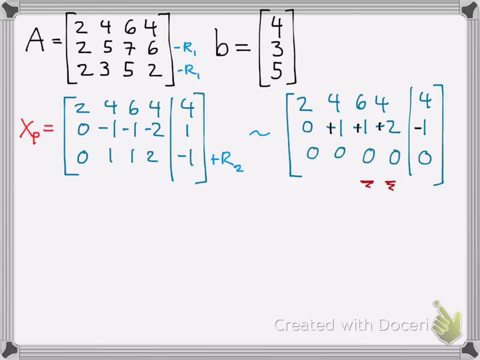 Again, that's just row reduction. should be plain and simple. Now, those two columns right there, those are free columns and in them, in and of itself, are the free variables X3 and X4,, those are free variables. 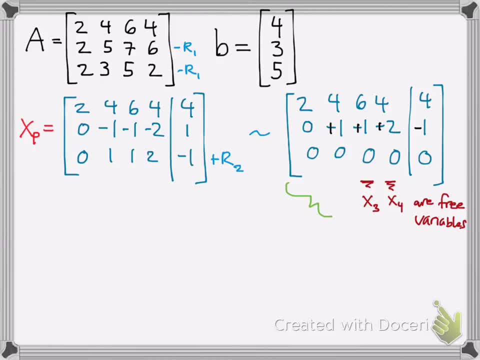 Now what we're going to want to do is set all our free variables equal to 0. But first let's write out the equations. The matrix represents a system of equations, right? So I wrote out the equations for those lines, and then: 0 equals 0 would be the last one, but no need to write that. 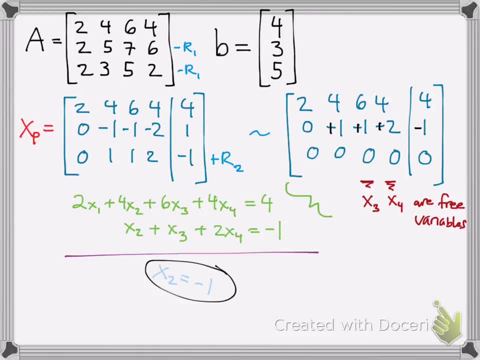 But we have our equations now. So once we set all our free variables equal to 0, so we're going to make X3 equals 0 and X4 equals 0. So look at the second equation. right now You have X2 plus X3 plus 2X4 equals negative 1.. 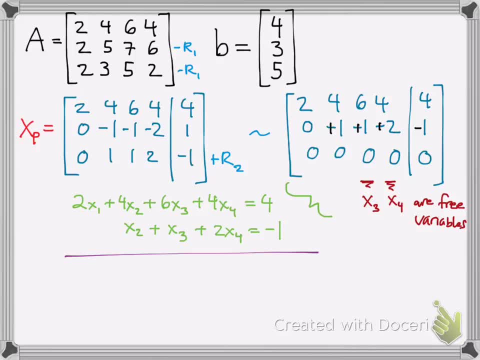 If we set X3 and X4 equal to 0, well, we would just have: X2 equals negative 1, right? So then plug that into the first equation there at the top and simply solve for X1, and you should get X1 is equal to 4.. 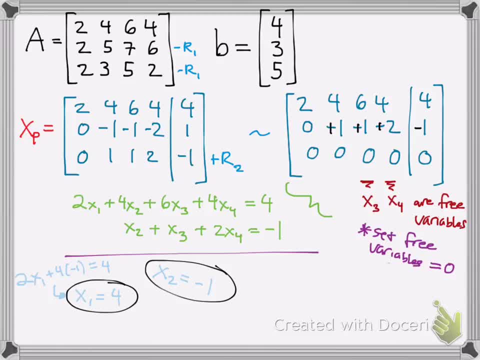 Well, that's what we got after. we set our free variables equal to 0, and that's how we find the particular solution. So our particular solution: well, we have X1,, we have X2,, we just solve for those. 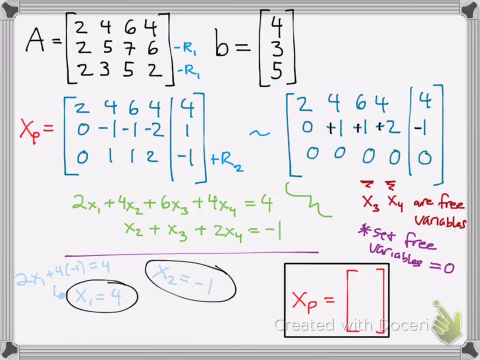 And what do we do with X3 and X4?? Well, we set them equal to 0. So we have 4, 1 should probably be a negative. Yeah, Hopefully that's fixed in the other video. It actually might not. 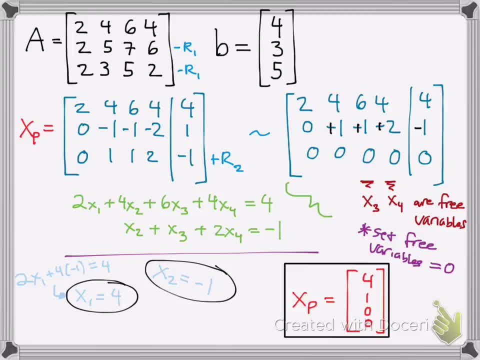 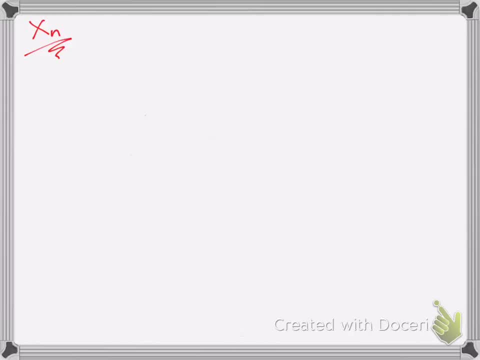 Oh wait, Is that right? Okay, That might be an error in the video. Keep that in mind. I'll see if I can go back to fix it at the end. Okay, So now we need to find Xn because, look, we found Xp right. 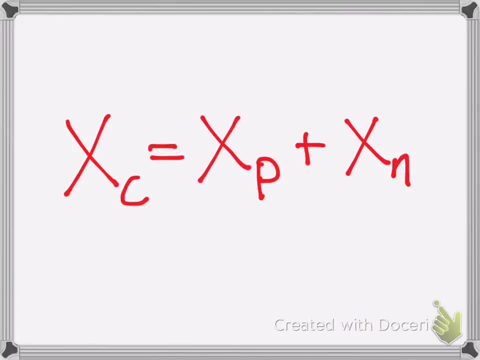 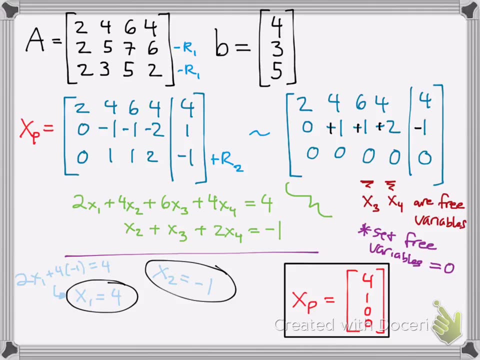 There's Xp, Now we're going to find Xn. So here's Xn. We're going to look back at the system of equations that we figured out down here. once we have the matrix row reduced, We're pulling out the equations, just what they normally do. 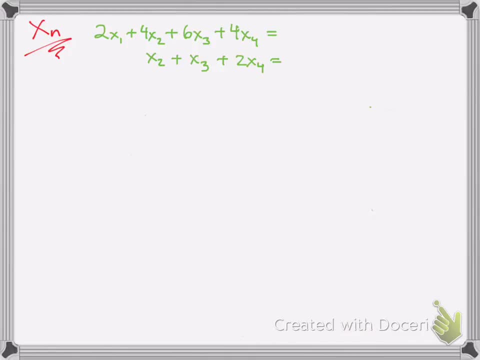 But instead of- since it's not augmented with the particular anymore, we're going to set those equal to 0.. Now solve for X2 in this portion And then you're going to plug it back in X1, just like you would normally do in any. you know first year algebra course, when you have a system of equations. 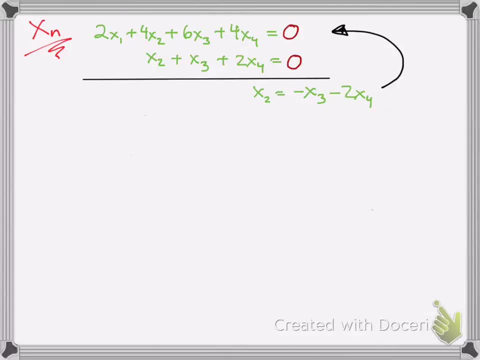 And you want to substitute your variables. You just do basic substitution here, Solve, Plug in the values here You should get. You can follow my steps along here. I'm going to make this kind of quick because this is a long subject to find the complete solution: a long process. 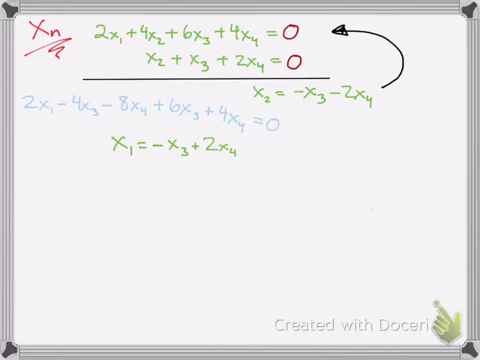 So then you should be able to get X1.. Now we have X1 and X2.. So again remember, X3 and X4 are free variables. So first let's see our template that we are going to create. 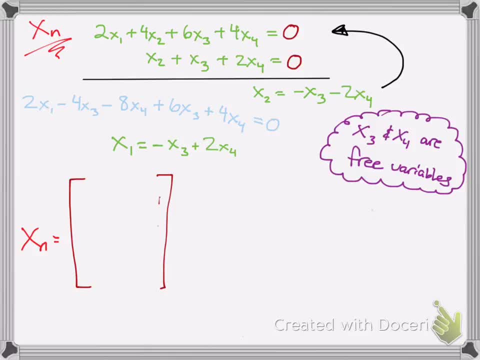 Kind of similar to what we did over here for our template, here for our special solutions. So X1 is what That's going to be the first spot there. That's negative X, That's negative X, That's negative X3 plus 2X4.. 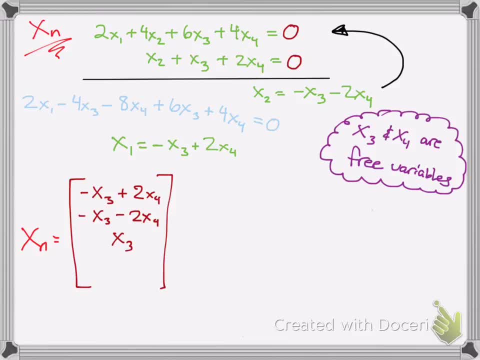 Then our X2 was negative: X3 minus 2X4.. And remember, our free variables are just our free variables. We're just going to list them there because they can be any arbitrary number that we want. But in order to find the special solution for each column space, what we're going to do is we're going to set each free variable equal to 1.. 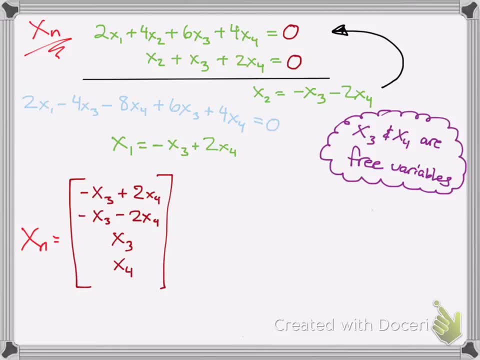 And then the other free variable is equal to 0. So set one free variable equal to 1 and the other to 0. So let's let X3 equal 1 first and let X4 equal 0, the remaining free variables. 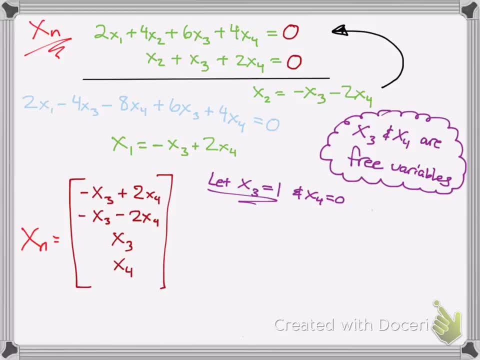 So all you do is plug X3 into the template over there on the left And then you'll have your special solution for the first column: space free column. space free column. So our first special solution would be negative 1, negative 1 and then 1, because that's what we let: X3 equal and 0.. 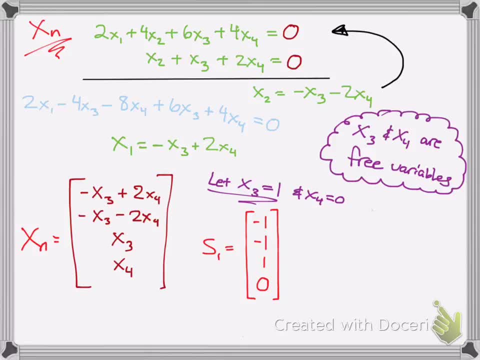 So again, just plug X3 into the template over there. Now we have: let's let X4 equal 1.. And let X3 equal 0. So now it's just flipping them. now So same thing We'll have: plug in X4.. 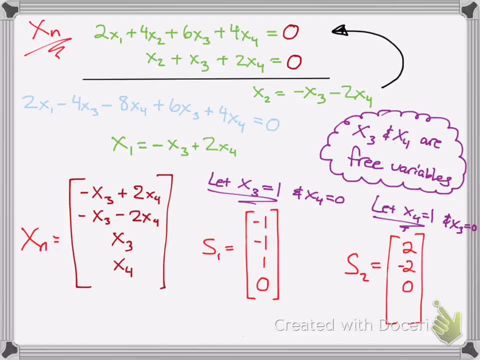 So we get 2 minus 2, 0, because X3 is 0 now, And 1,, which is what we need at X4.. So now we have our two special solutions. Okay, cool, We're done. 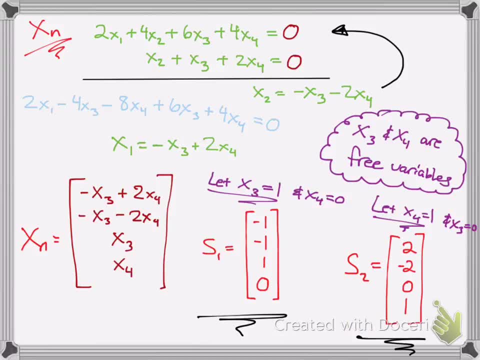 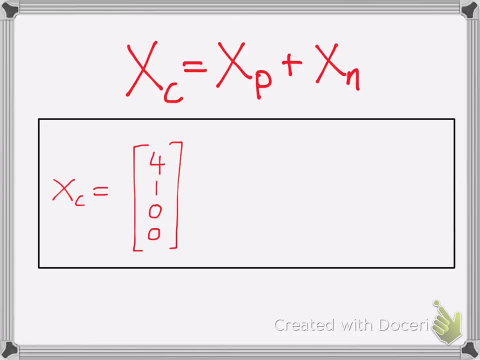 We have our particular solution- what we solved for here, and our special solutions. So let's put it all together now. So we have our complete solution- the particular, which is what we solved for here. Then we have our two special solutions- what we just solved for. 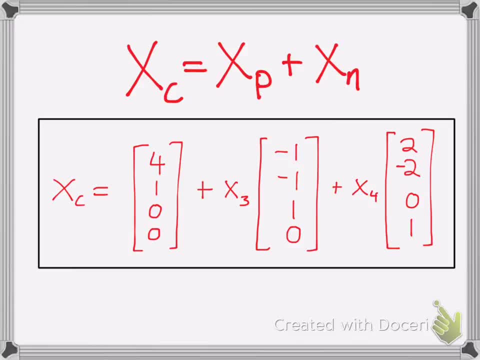 And there you have it. We have our complete solution now. So it's a long process to do it, but it's actually quite satisfying once you get it done and you figure out what you did. So this was the method on finding the complete solution in linear algebra.